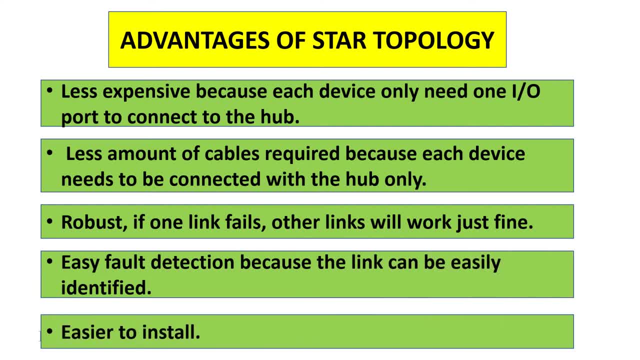 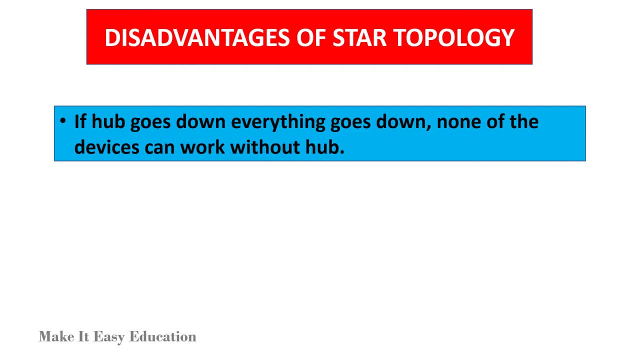 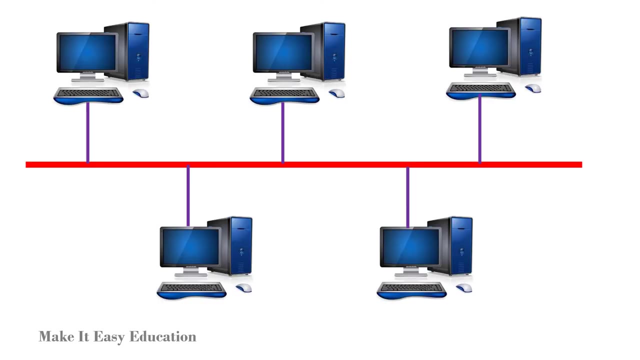 the link can be easily identified, easier to install. disadvantages of start apology: if hub goes down, everything goes down. none of the devices can work without hub. hub requires more resources and regular maintenance because it is the central system of start apology. bus topology. in bus topology there is a backbone. 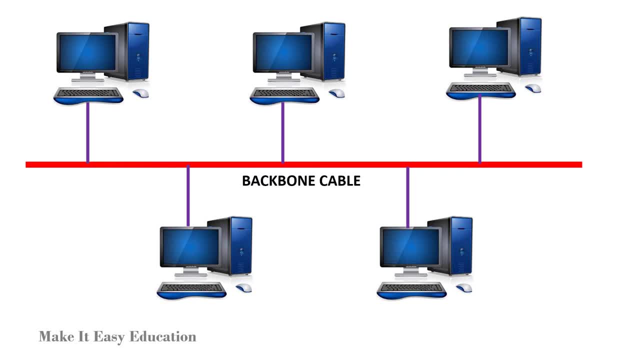 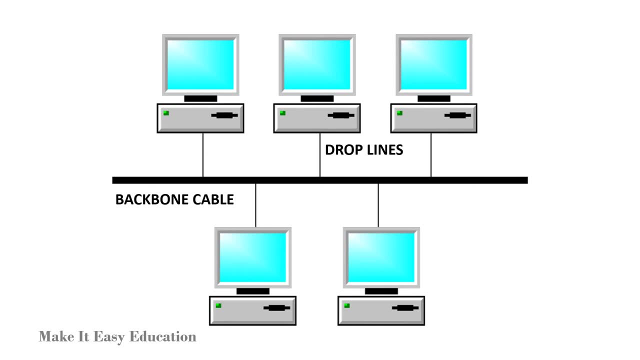 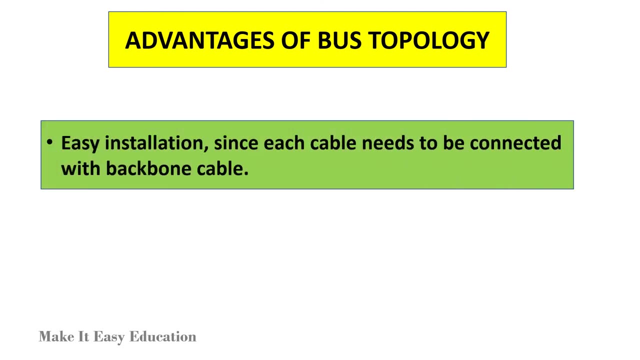 cable and all the devices are connected to this backbone cable through drop lines. since all the data is transmitted over the main cable, there is a limit of drop lines and the distance. the main cable can have advantages of bus topology. easy installation, since each cable needs to be connected to the main cable. the main cable needs to be connected to the. 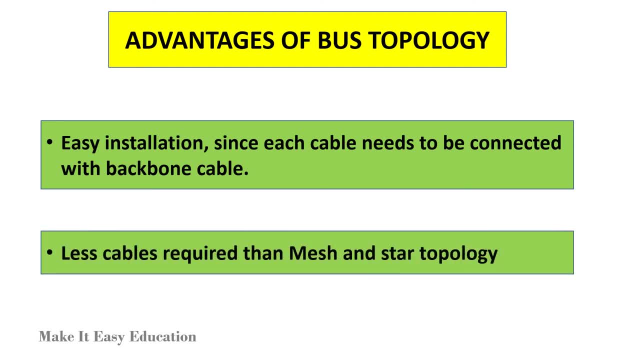 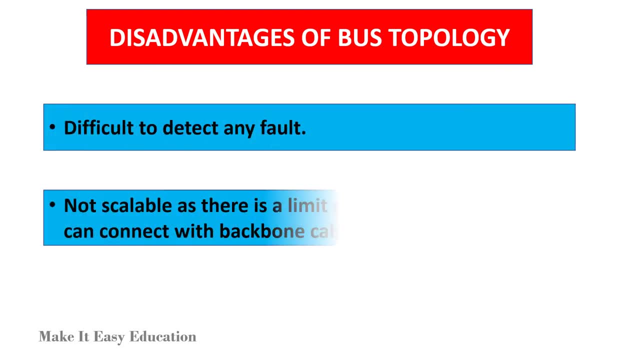 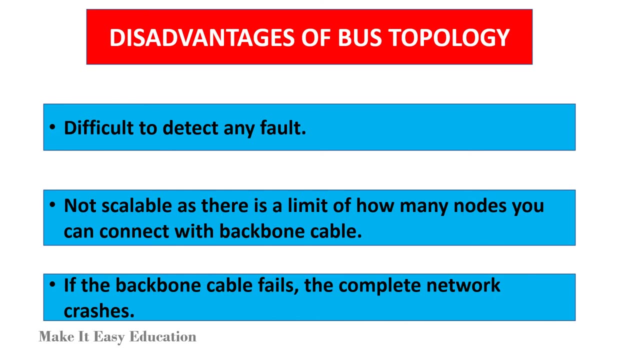 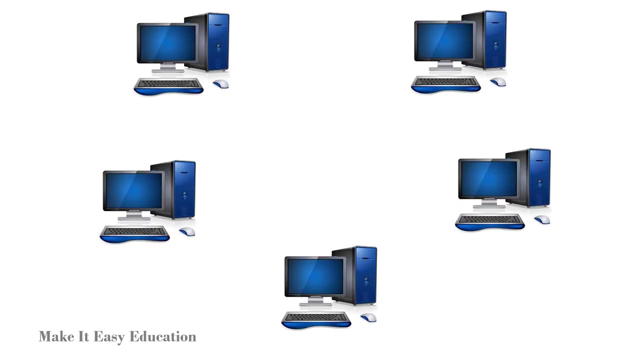 backbone cable. less cables required than mesh and start. apology: disadvantages of bus topology. difficult to detect any fault. not scalable, as there is a limit of how many nodes you can connect with backbone cable. if the backbone cable fails, the complete network crashes. ring topology: in ring topology each device is. 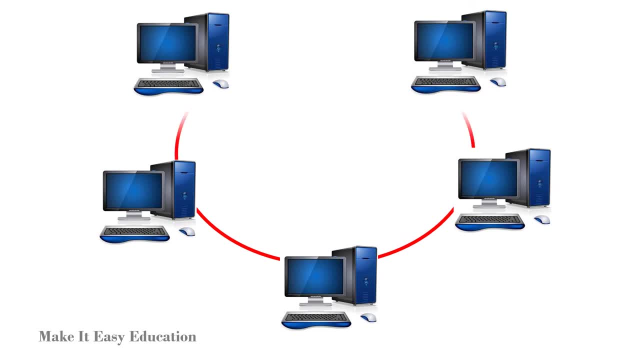 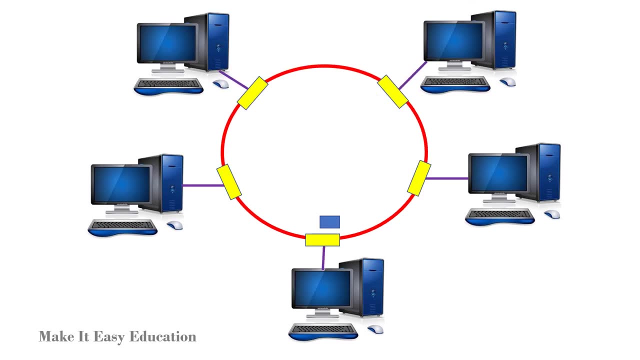 connected with the two devices. on either side of it, this structure forms a ring. thus it is known as ring topology. each device in ring topology has a repeater. if a device wants to send data to another device, then it sends the data in one direction. if device one wants to send data to 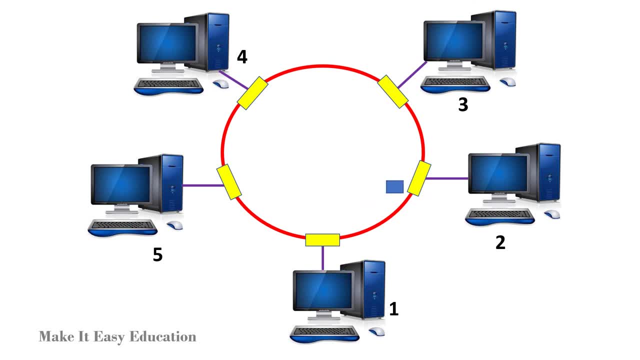 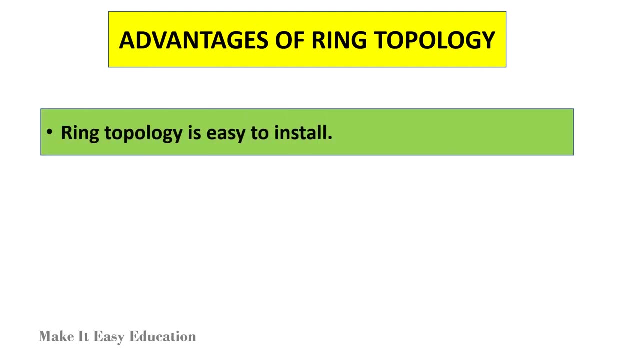 device five, it first sends the data to device two. if the received data is intended for other device, then repeater forwards this data until device five receives it. disadvantages of ring topology. ring topology is easy to install. managing is easier. as to add or remove the device from the topology, only two links are. 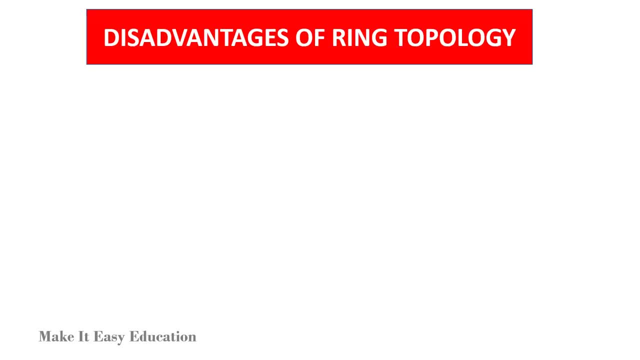 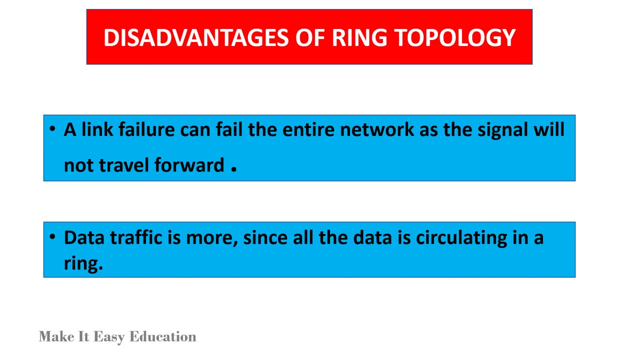 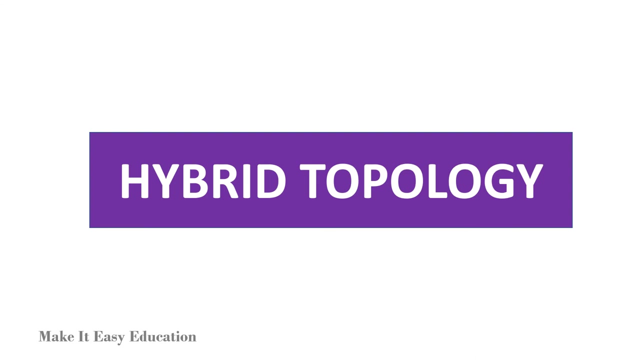 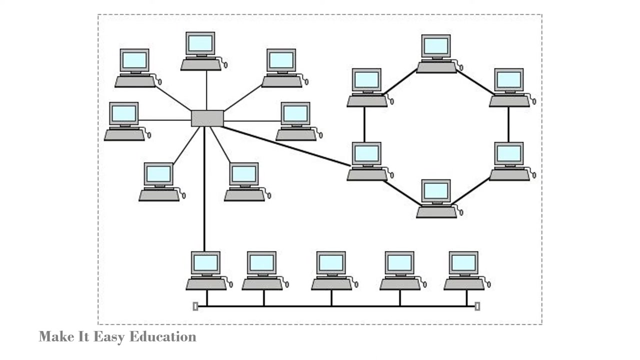 required to be changed. disadvantages of ring topology: link failure can fail the entire network as the signal will not travel forward. data traffic is more, since all the data is circulating in a ring. hybrid topology: a combination of two or more topology is known as hybrid topology. for example, a combination of: